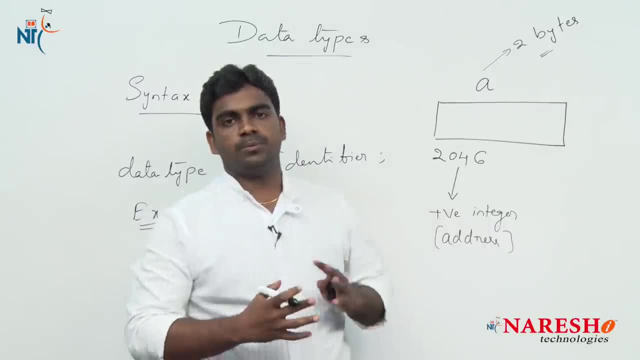 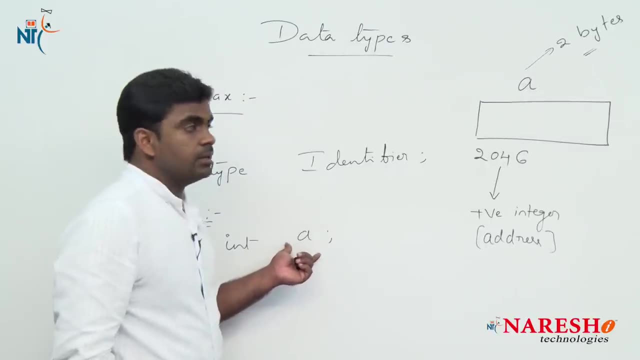 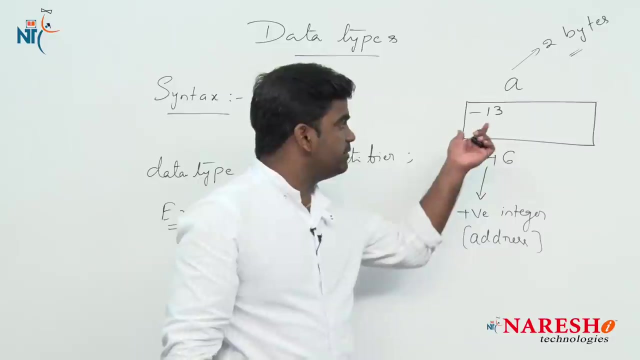 another variable goes to production. Okay, So again, what we will do is, once data type is stored, we will add data. This is your code string, right, And you will see so many к forever. this Suppose, here it is, I am storing. minus 13 is a negative integer. of course it is an integer. 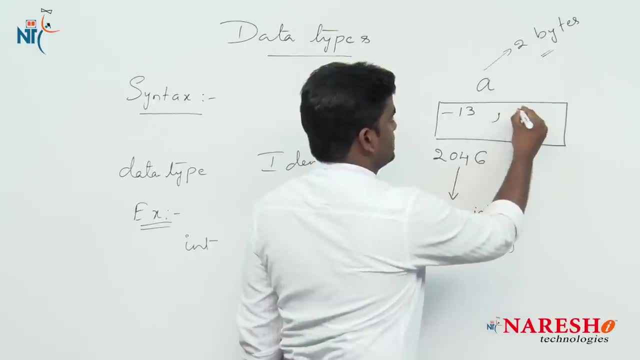 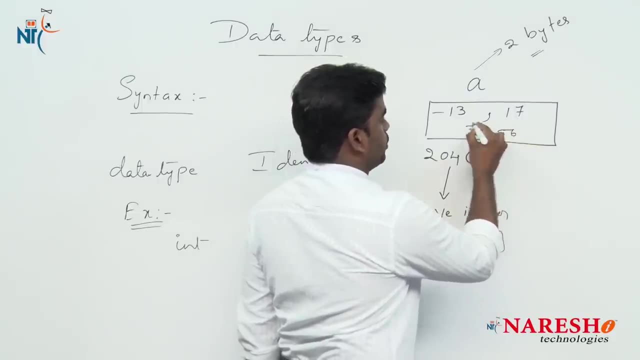 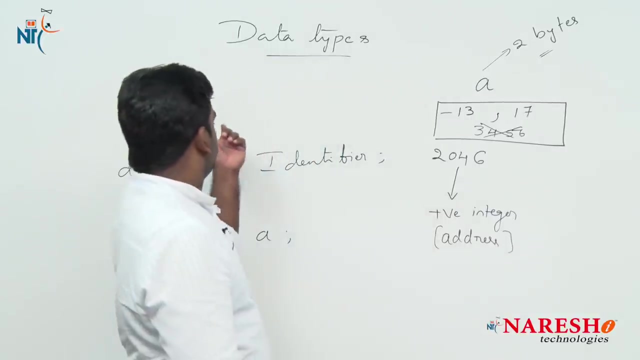 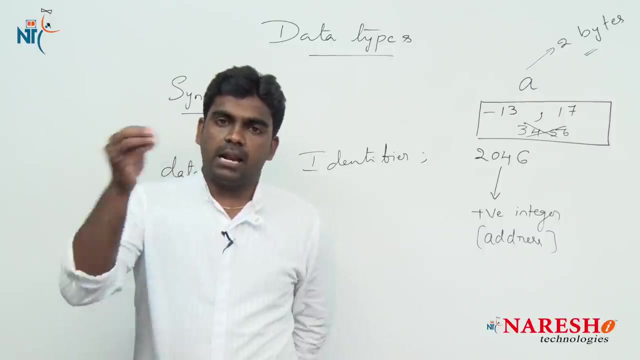 so it is allowed. and next one, some positive integer 17 I am storing. it is also allowed. but can we store a 34.56? no, it will not allow decimal values. not allowed, simply, data type represents two things about a variable. first one: what type of data is allowed to store? 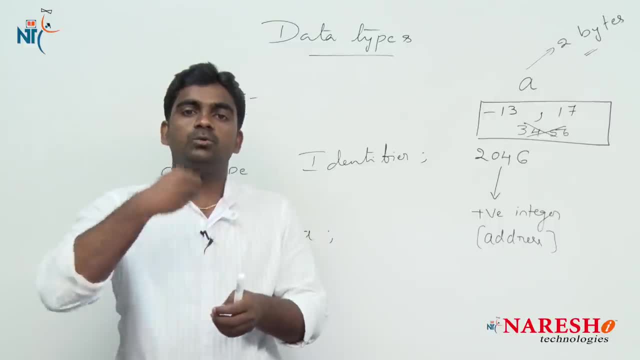 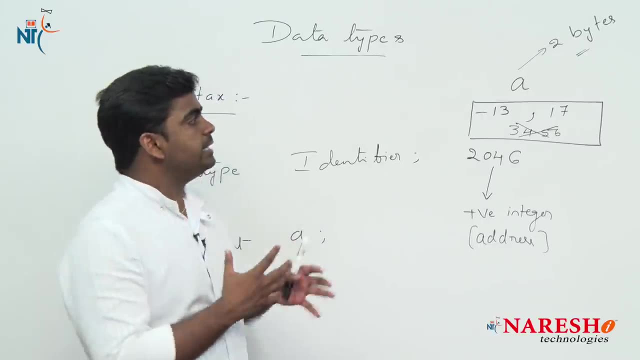 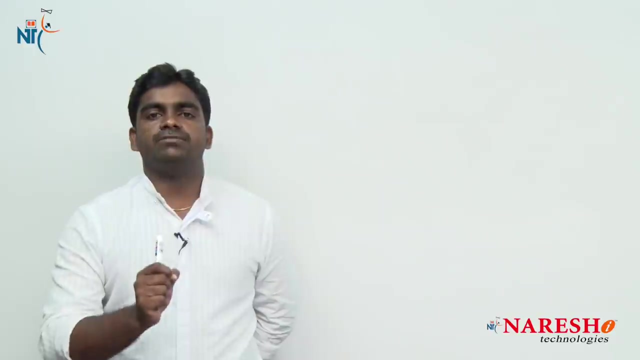 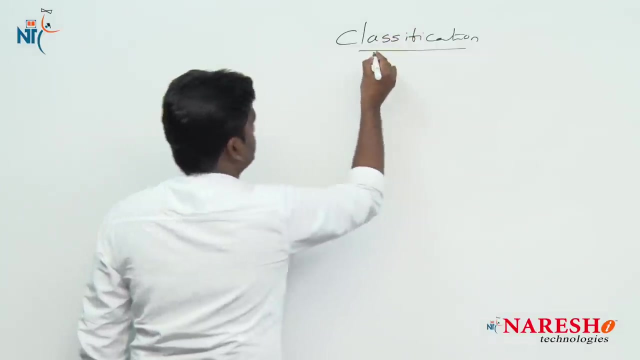 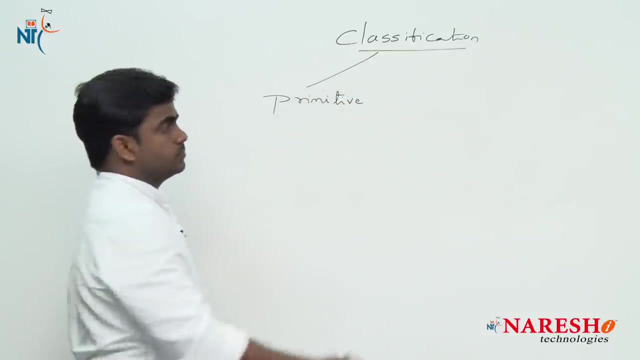 and second one: how much memory is required to store the data, these two things so described by a data type. and now how many types are available in a C language? ok, C, here it is data types classified into three types. Classified into Three types. this is a classification. so first one, primitive data types. second, one derived. 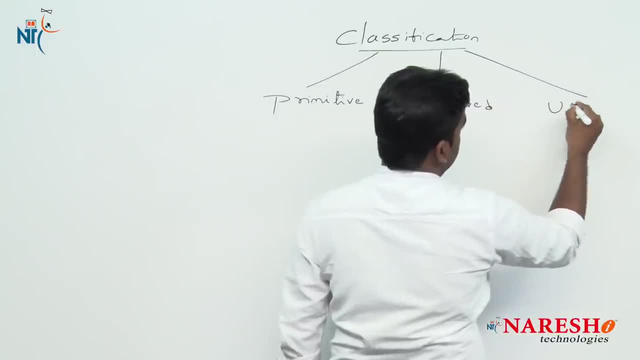 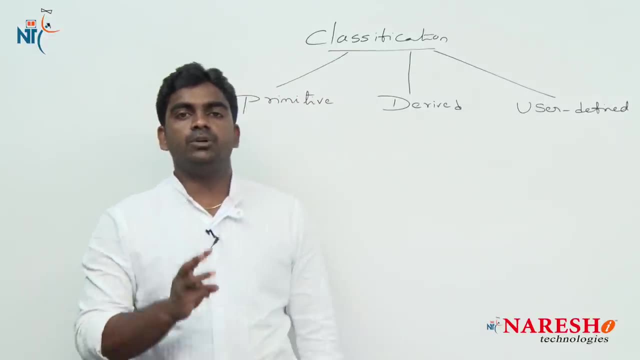 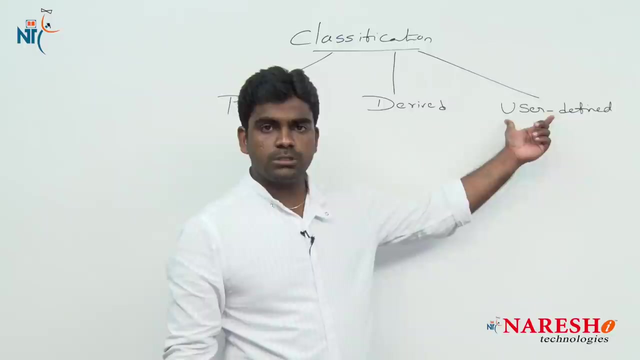 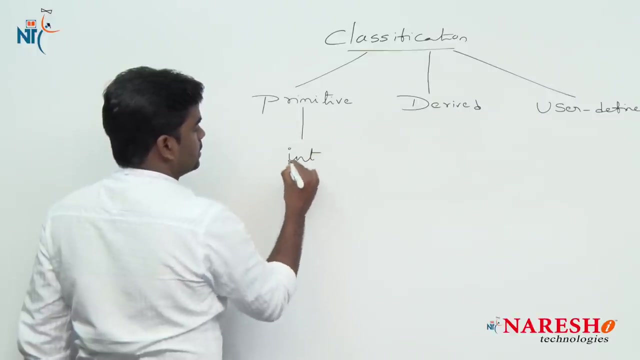 data types. third, one user defined data types. data types classified into three types. first one is a primitive data types. second one is a derived data types. Third one is a user defined data types. right here it is a primitive data types. integer, character, float, void- all these are called primitive data types. these are comes under. 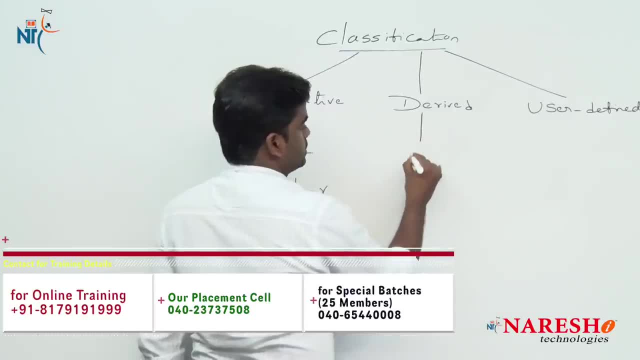 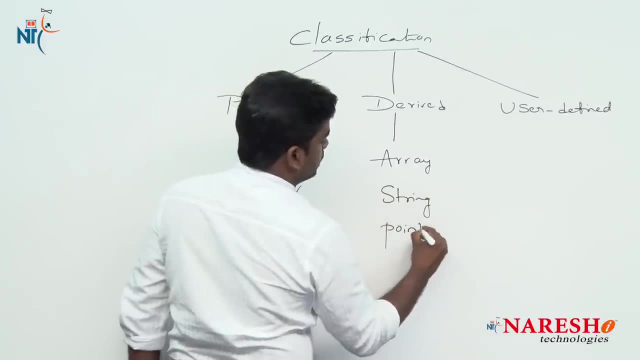 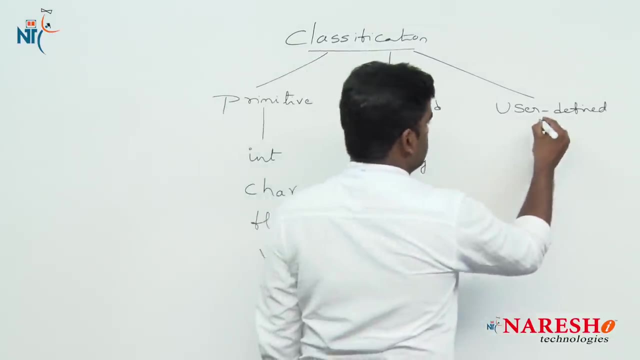 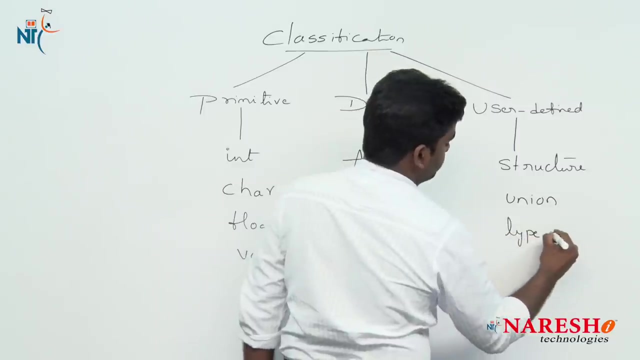 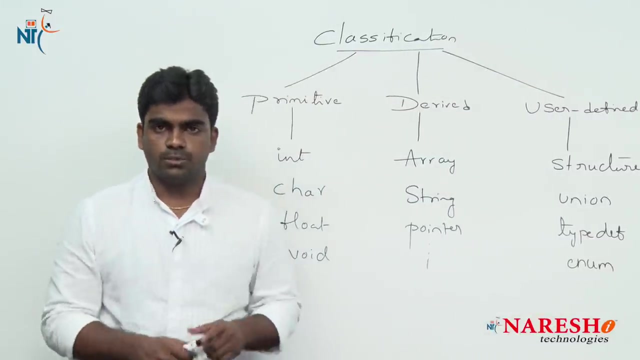 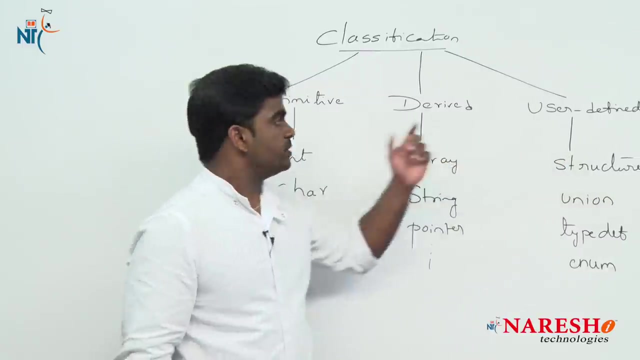 primitive types. what are the derived types? suppose array, string, pointer, all these are under derived data types. And what are the user defined data types? Here it is structure, union, typedef, enum. All these are comes under user defined data types. So, once again, data types divided into 3 types, classified into 3 types. First, one primitive, 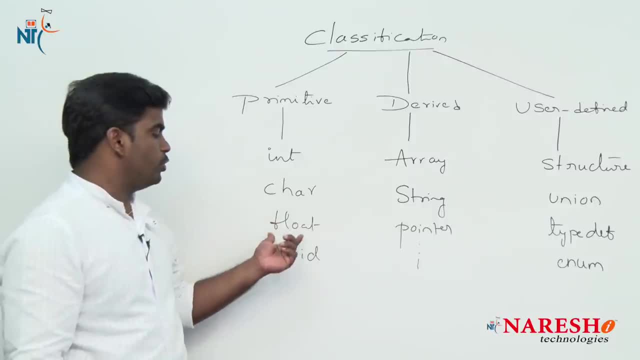 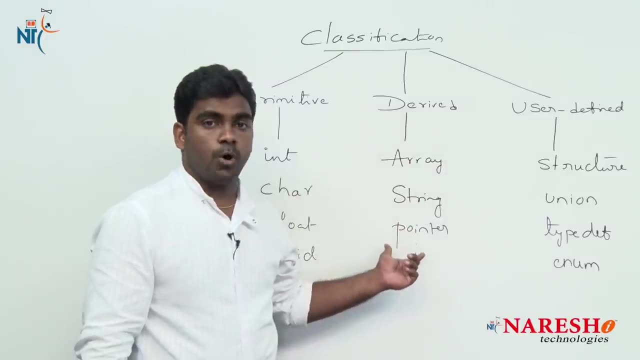 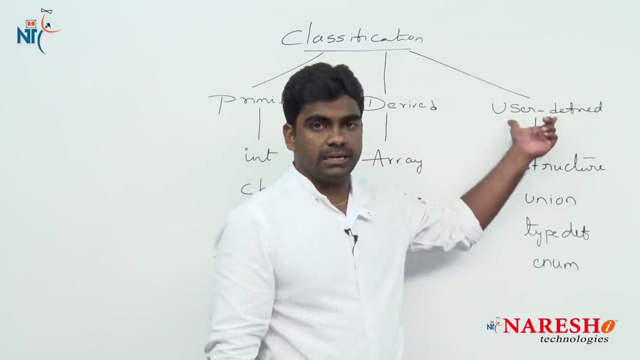 data types: integer character, float void. Second, one is a derived data types. arrays, strings, pointers, functions and all these are comes under derived data types. And what are the user defined data types? Structures, unions, typedef, enum. So 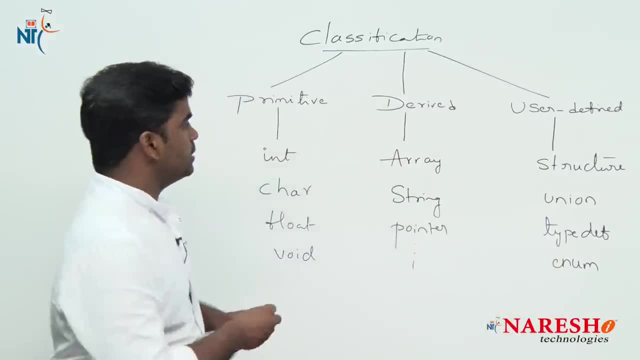 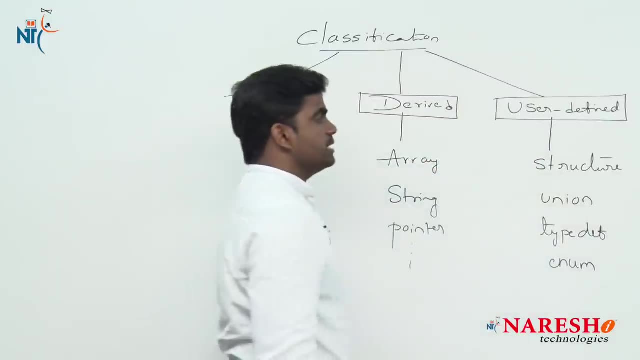 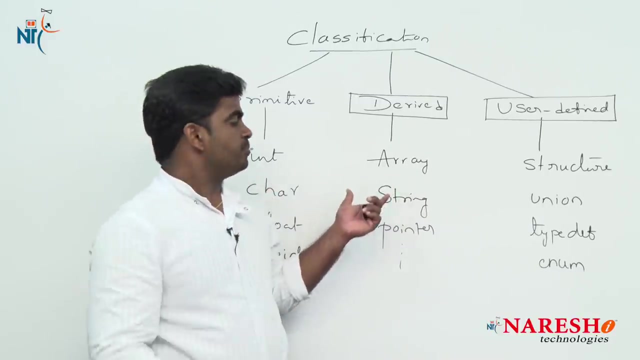 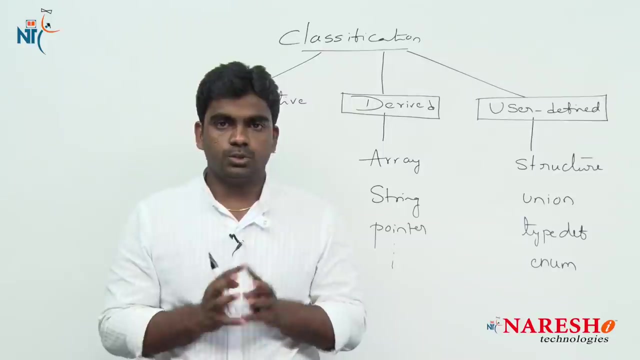 this is called classification And here either derived data types or user defined data types. These data types discussion later. So because arrays we will discuss very clearly as a concept And strings also we will discuss Structures, unions. all these are separate concepts in a C language, So data types means only just. 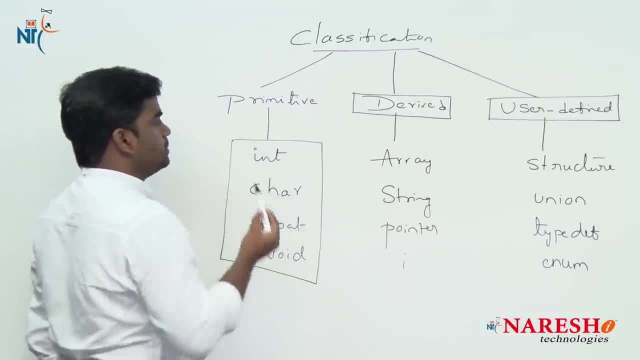 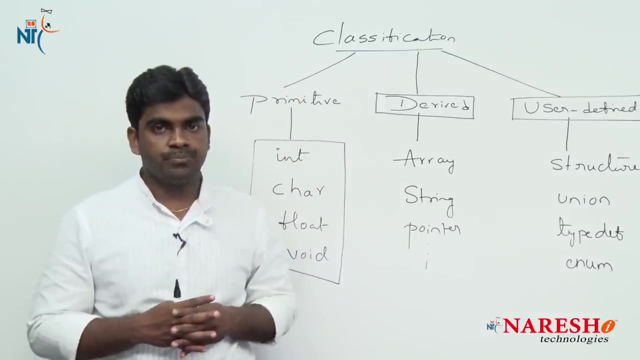 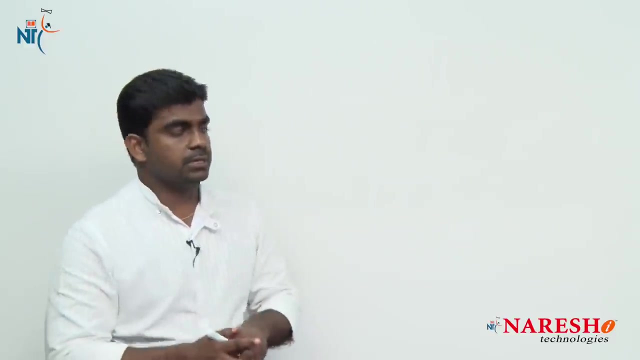 these primitive data types discussion. So first, primitive types, again subdivided into so many data types. So what are the types We will see? So, sub classification of primitive data types Here, primitive types only. And what are the primitive types? Once again, we are writing. 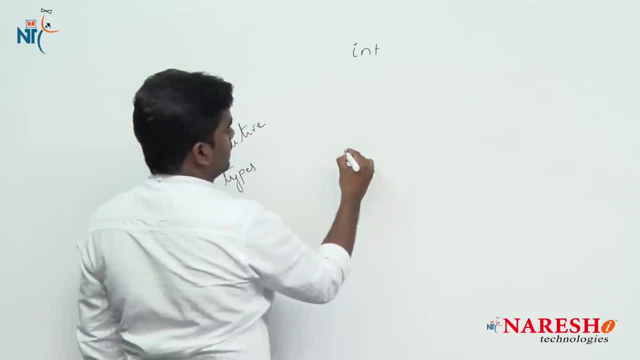 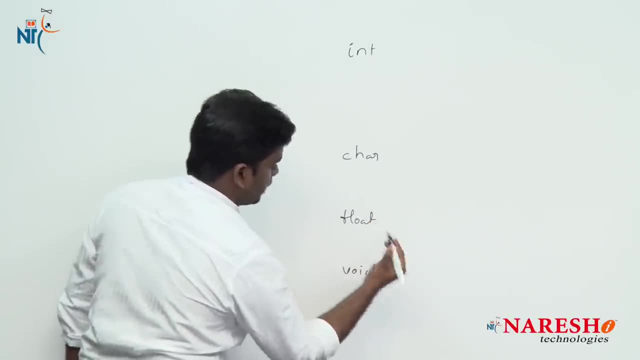 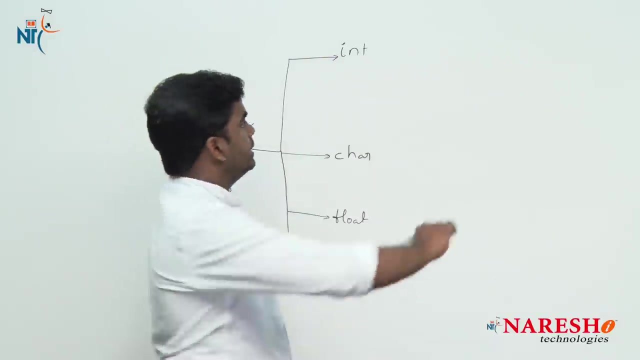 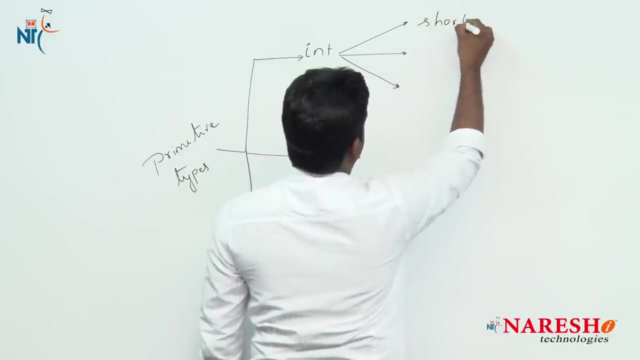 integer, next one character, next one float and the last one is a void. So these are the primitive types. And what are the integers types? Integer divided into three types. First, one is a short, Second one is integer. 3rd one is a long. 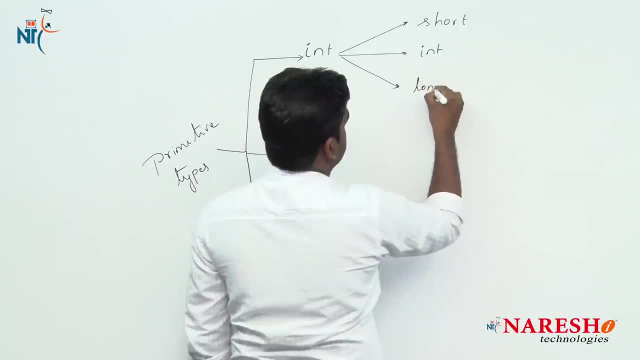 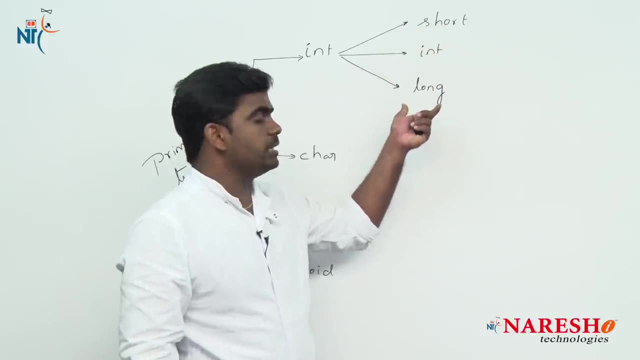 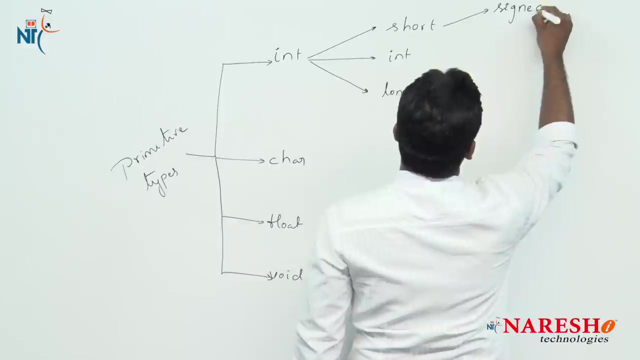 First one is a short type, Second one is integer, third one is a long. First one is a short type, second one is an integer and third one is a long And again a short. data type divided into two types. One is a signed short. 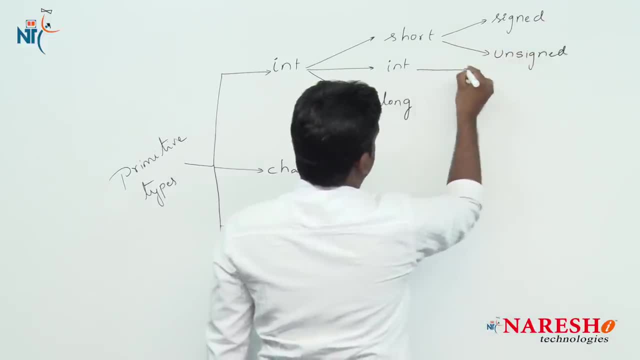 second one is aadesh and second one is a pull. And what are the integer types? And what are the integer types? Integer divided into 3 types. one is a unsigned short Integer. also one is a signed integer. second one is a unsigned. 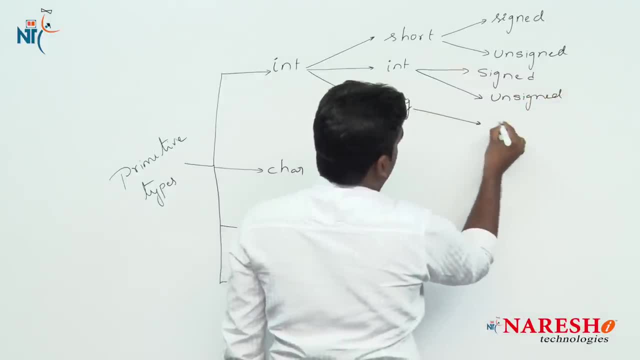 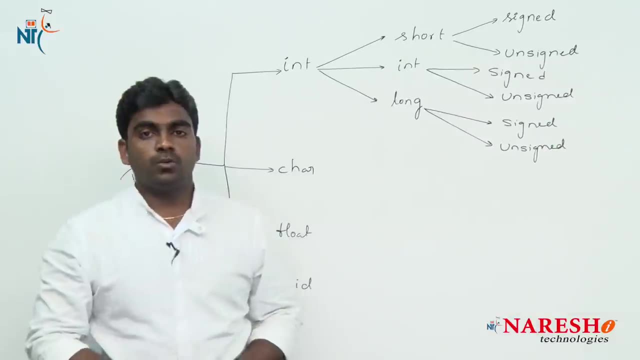 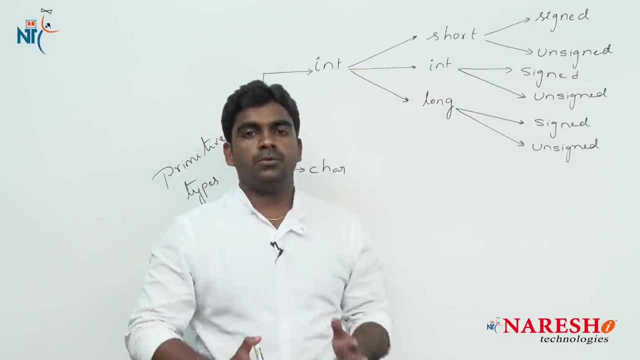 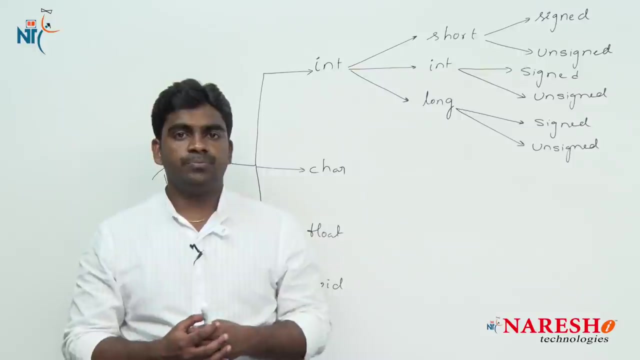 integer Long. also, one is a signed long, second, one is a unsigned long. So one integer data type, again subdivided into six types, Sir. why, sir, Suppose, if you want to store one integer value, right, one integer data type is enough. na Why these many data types? 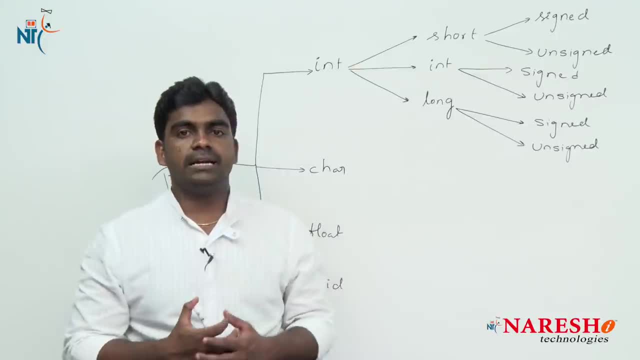 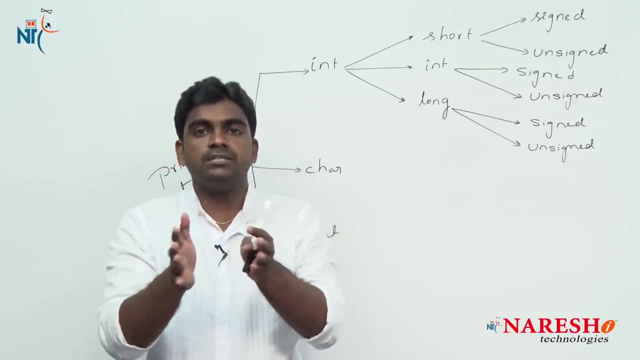 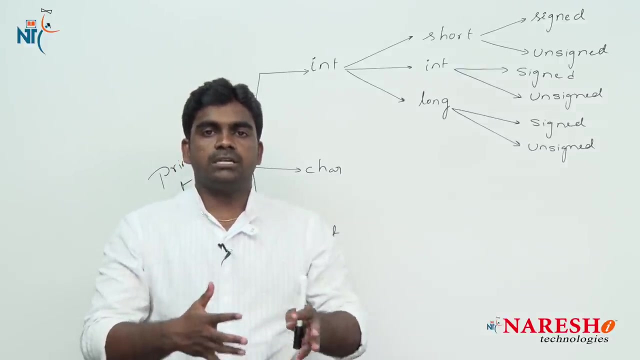 are required. Why these many data types are required. Why again classified into six types? Depends on the data we are storing, depends on the size of the data. I just want to store the balance in a account- 5000,, 6000, then we choose one particular type, For example: 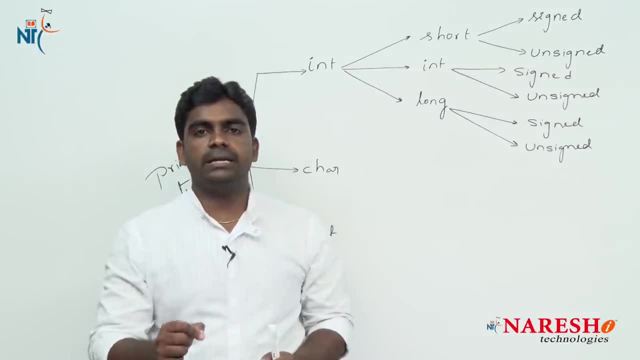 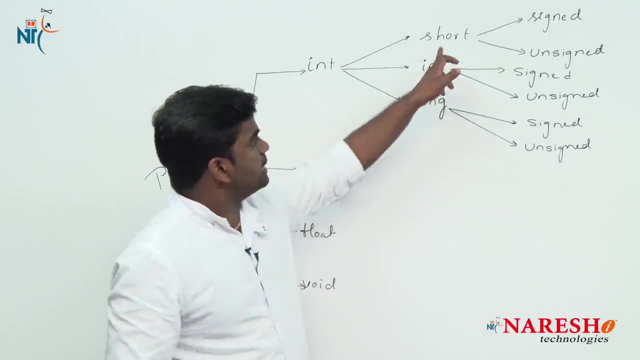 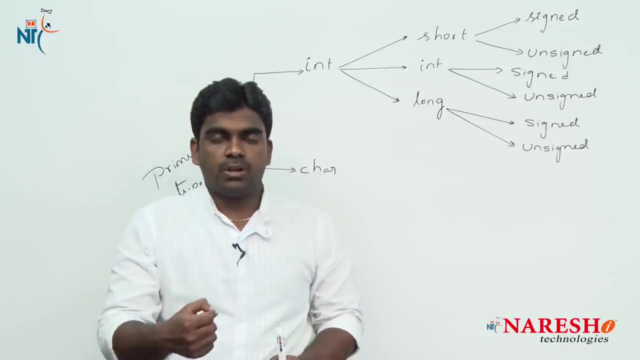 department number, So mostly 30,, 10,, 20 department numbers are there right To store such type of data. so very a less integer is enough, For example short. Just consider I am trying to store a phone number or I am trying to store account number, right, Such type of things we can store. 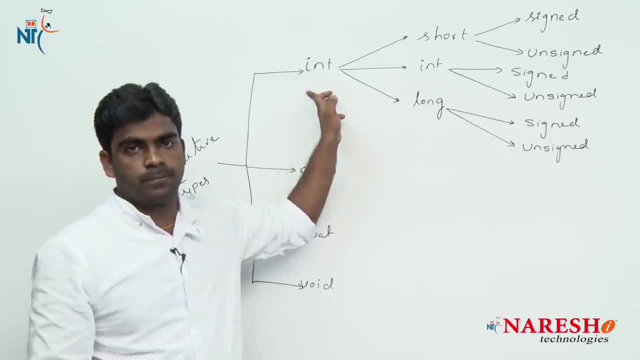 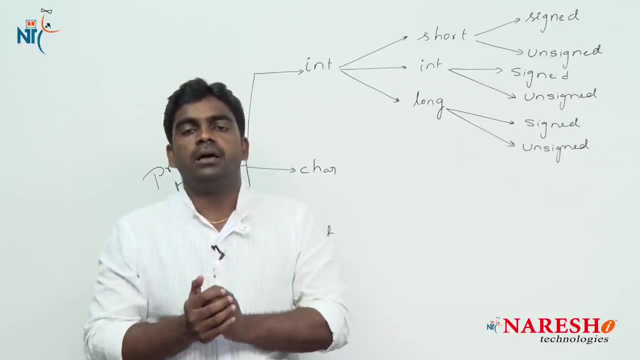 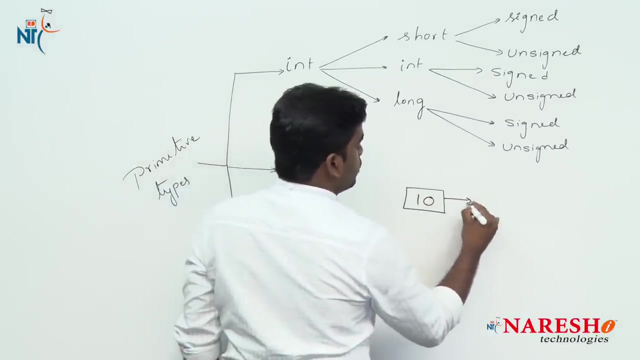 with the help of only long integer types. only Depends on the size of the data right. We choose a particular data type right among available. For example, suppose 10.. To store the value 10, 1 byte memory is enough: 1 byte. 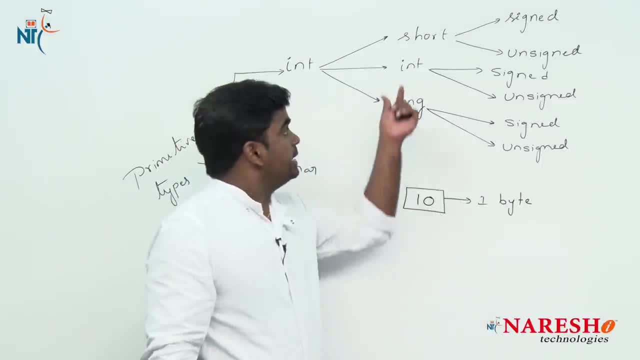 memory. So always we should go for a data type which occupies only 1 byte memory. Suppose if you are trying to store a table which translates into only 1 byte memory, those tables can kinda be filled-in This same table too. So always when you go with work then this whole table is one pinch. that denotes: 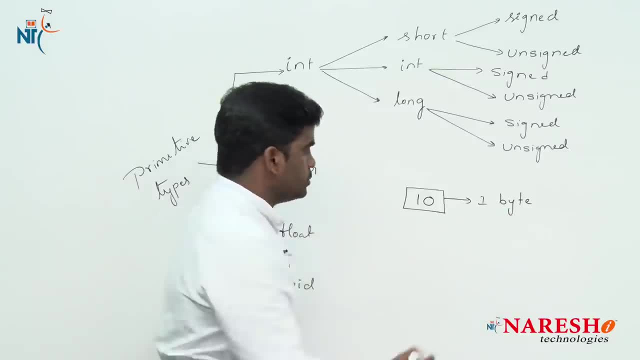 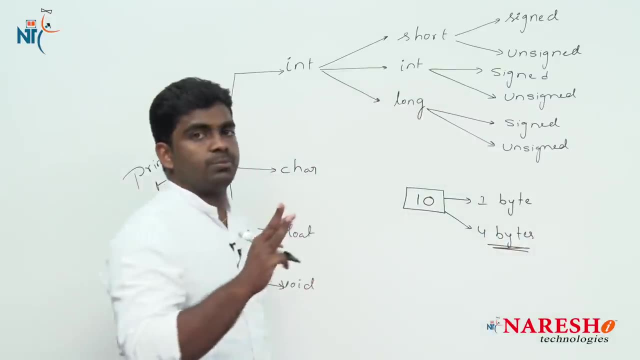 by which you storage data type and then occupies only 1 byte memory. suppose if you are trying to choose a, a data type which occupies 4 bytes, wantedly, you are wasting 3 bytes memory in your application. 3 bytes of memory we are wasting. 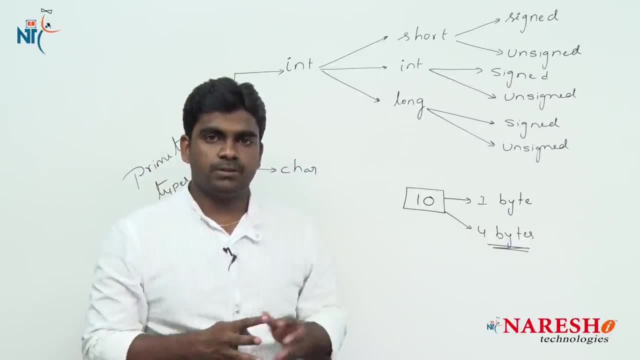 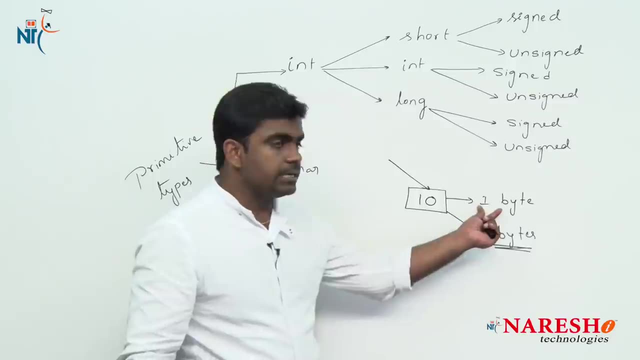 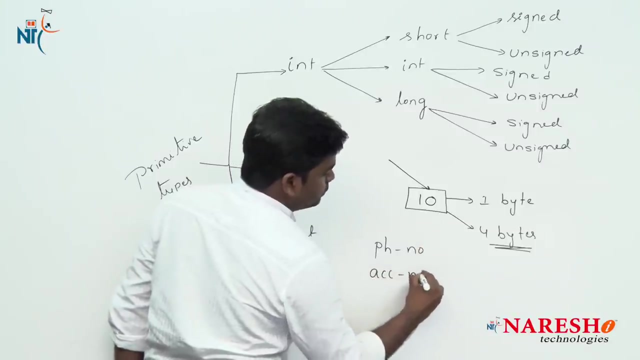 So that reduces the application performance. so that is why always depends on the data we are using or we are storing, right, we should select a particular data type. suppose I am storing a phone number or I am storing an account number, then we should go for the data. 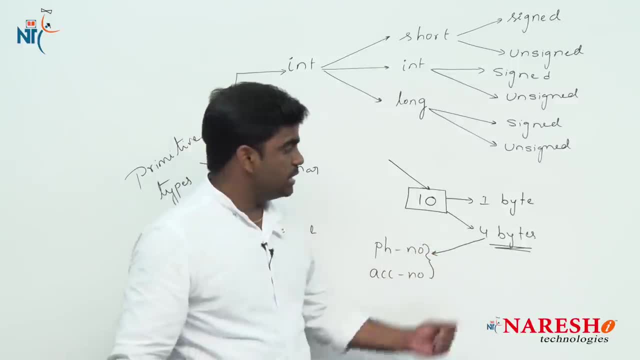 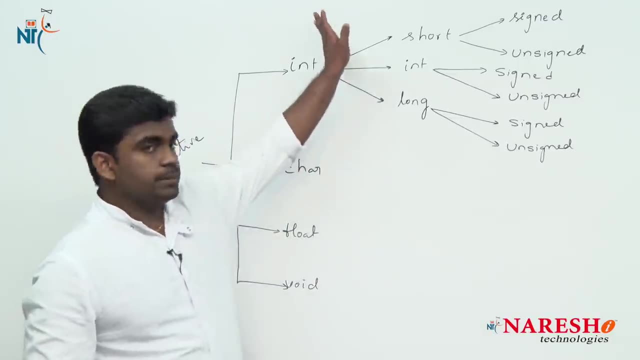 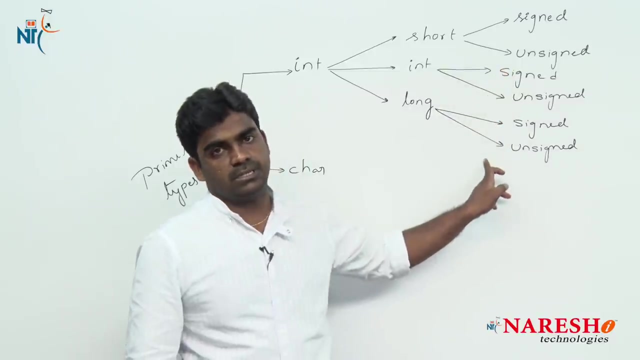 type which occupies 4 bytes memory, because 1 byte memory is not enough to store such type of informations. So this is integer types and how to select a particular type and why they divided 1 integer type into 6 subclassifications And next character character, also divided into 2 types. 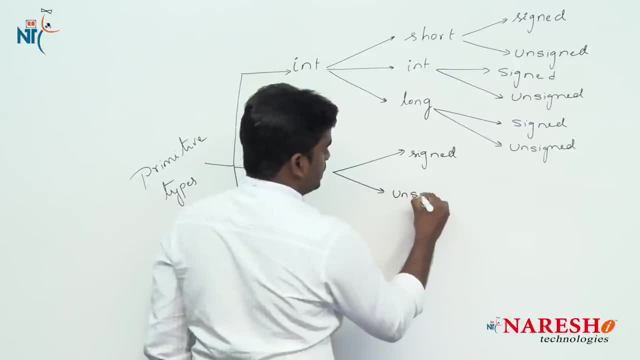 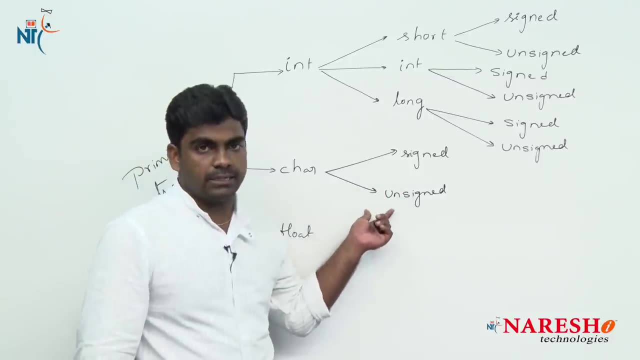 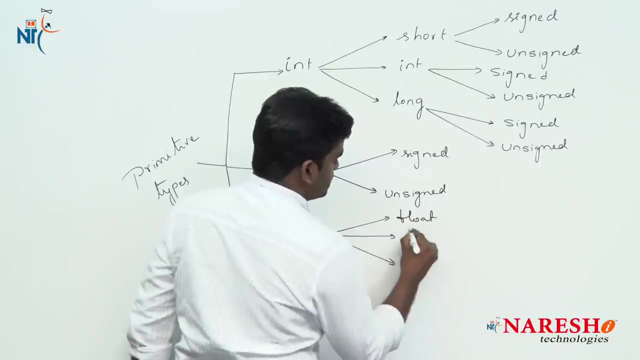 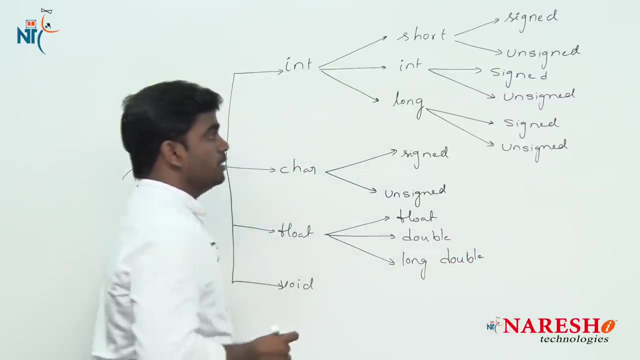 One is a signed character and second one is a unsigned character. one is a signed and second one is a unsigned character and next one float, divided into 3 types. one is a float type, second one is a double and the last one is a long double. last one is long double. 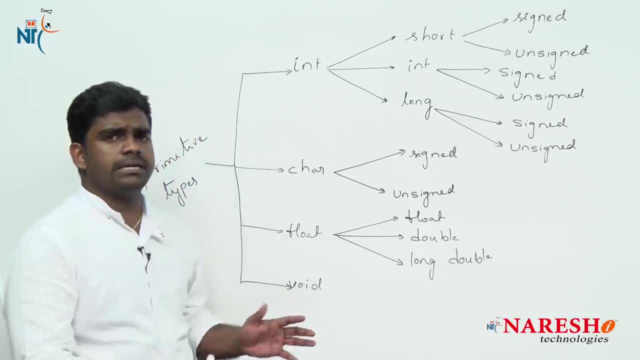 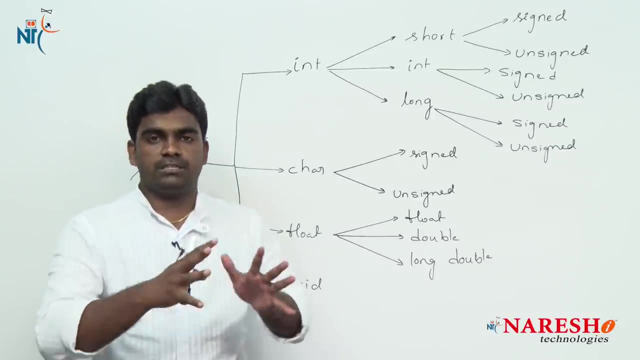 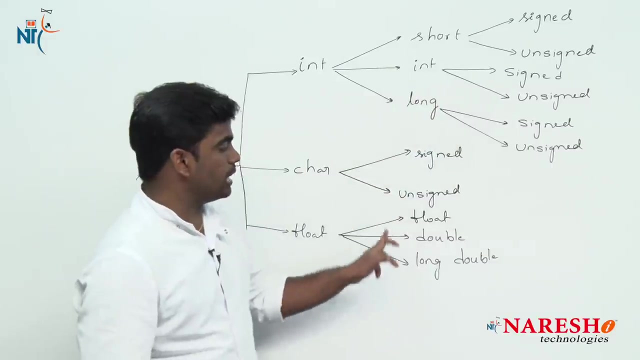 So these are the classifications. Wide just, it is representing nothing thing. and more clearly, once already we discussed and once again we will see more briefly in a functions concept. So here it is, a 3 types, 3 types again subdivided into. so total, how many types? 11 types. 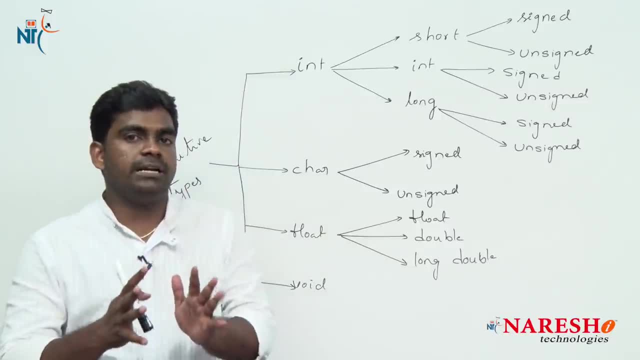 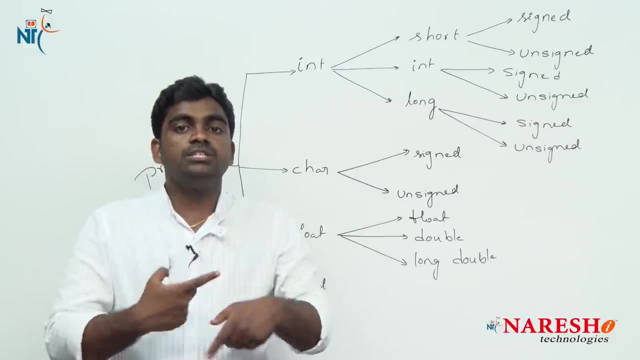 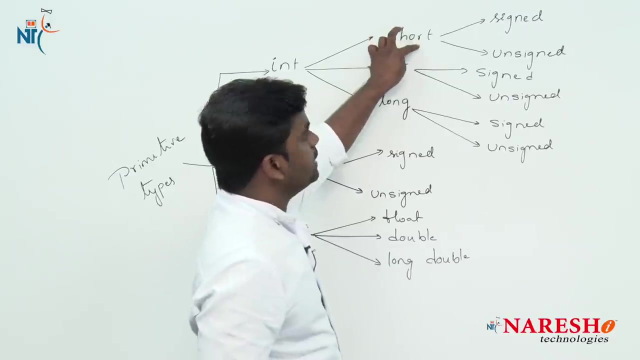 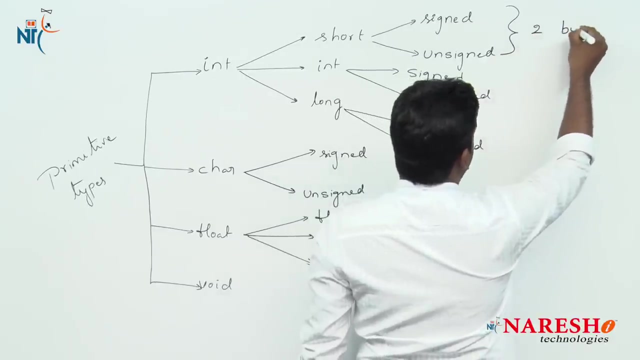 So this is called a sub classification of data types. sub classification of data types and after that how many bytes each data type occupies. How many bytes each data type occupies, see suppose, if it is a short integer, either it is a signed integer or it is a unsigned integer. it occupies 2 bytes memory in the program. 2 bytes memory in the application and suppose if it is a integer right, either it is a signed or in unsigned, it will occupy 2 or 4 bytes. sir, when it will occupy 2 bytes and when it will occupy 4 bytes, That is depends on the compiler we are using that. once again, we will see briefly right. 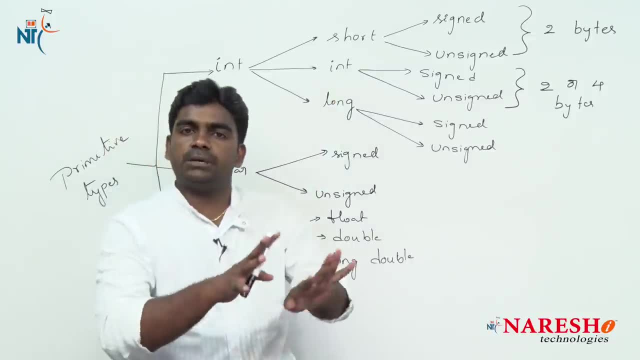 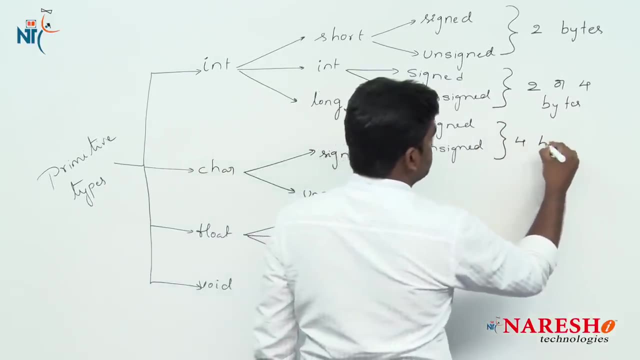 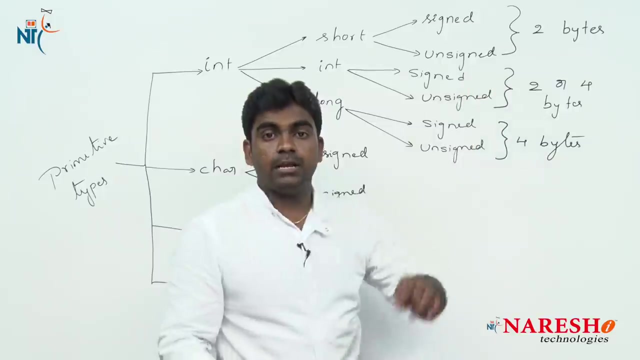 when we are going to discuss about a integer data type, particularly ok. And next, long right: either signed or unsigned. it occupies 4 bytes memory. once again, short data type. either it is a signed or unsigned. again, questions are: what is a signed and what is unsigned? simple. 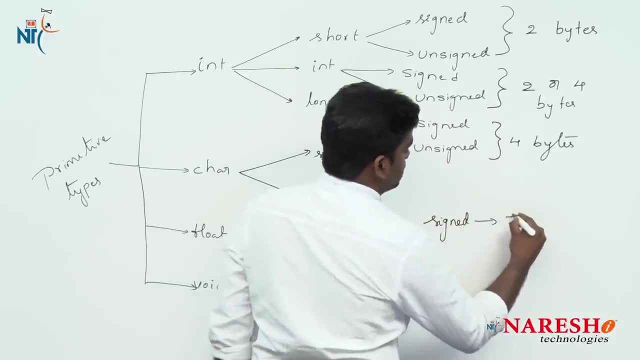 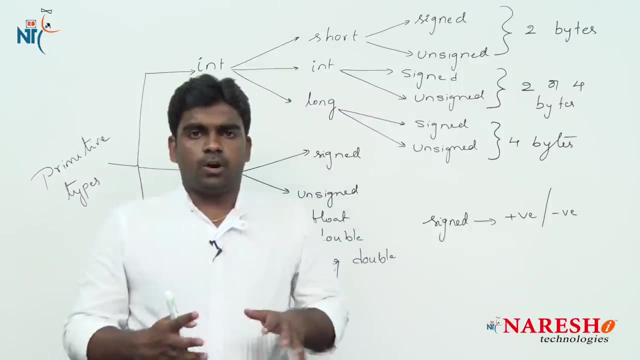 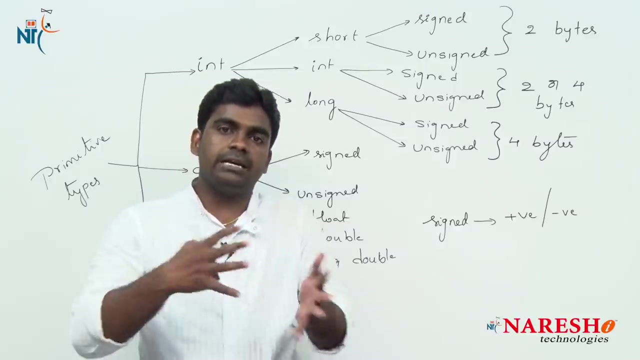 Signed means Using signed data type. we can store a positive value or negative value. both are allowed in our program always. we are not working with only positive values. in some of the cases definitely there is a requirement will come that we have to store negative values also. 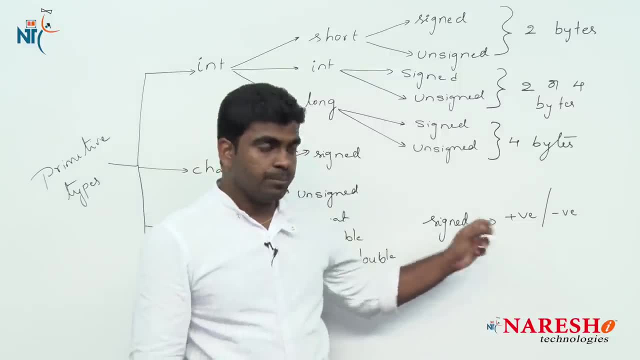 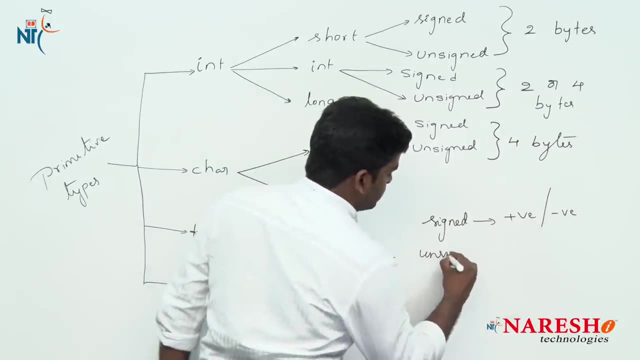 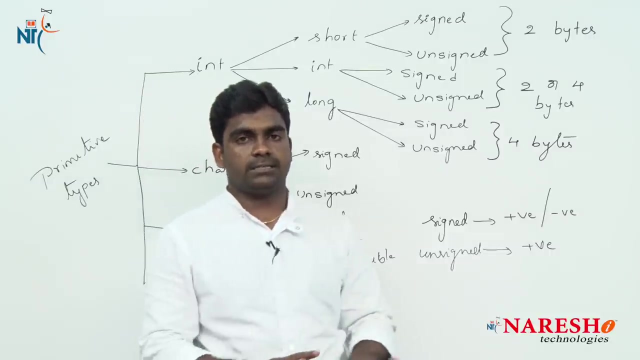 in that situation we should go for signed type, because a signed data type accept both a positive value and a negative value. But suppose if it is a unsigned type, Unsigned Strictly, it will accept only positive values, negative values it will not accept, right? So this is a difference between signed data type and unsigned data type. here it is short, either it is a signed or unsigned. it occupies 2 bytes. integer, either signed or unsigned. it occupies 2 or 4 bytes depends on the compiler we are using, and if it is a long it occupies. 4 bytes. Character: Either signed care or unsigned care. it will occupy only 1 byte memory. it will occupy only 1 byte memory and next one. float data type occupies 4 bytes. double data type occupies 8 bytes long. double data type occupies 10 bytes memory. in the application right.